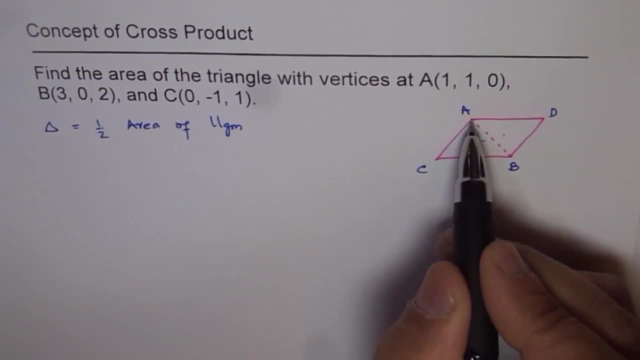 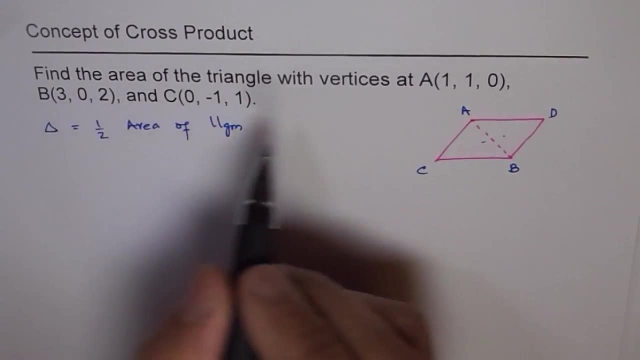 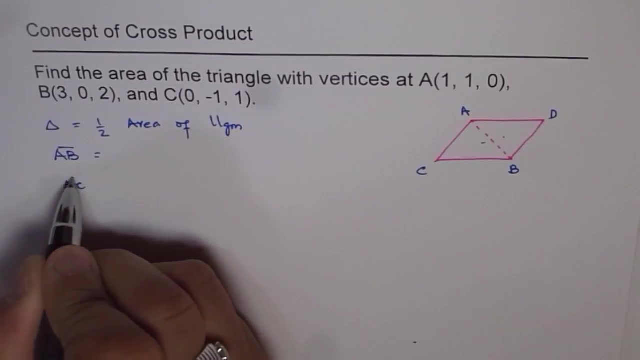 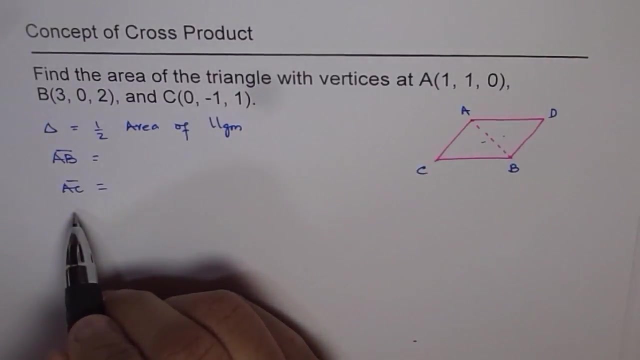 And what is area of parallelogram? Area of parallelogram will be cross product of two sides, correct? So what we will do here is we'll find the two sides, which is AB and AC. So once we have two sides, let's say AB and AC, then we can do cross product of AB and AC and half of that and its. 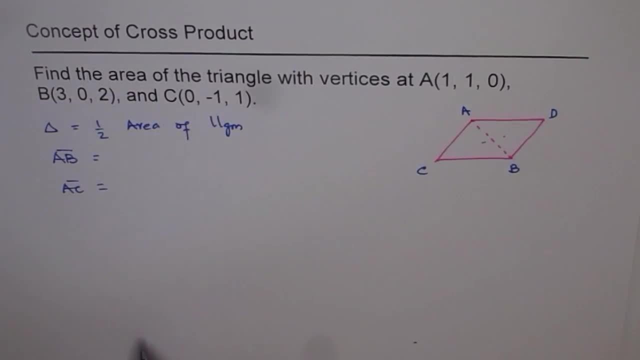 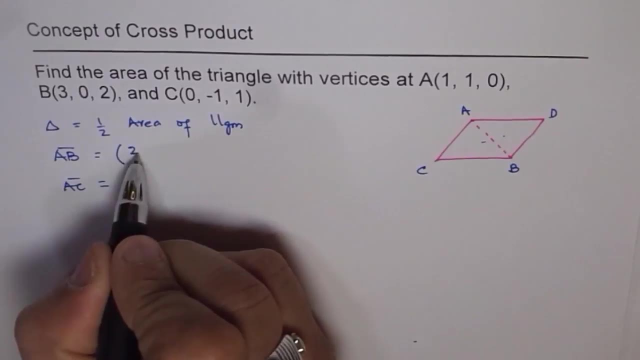 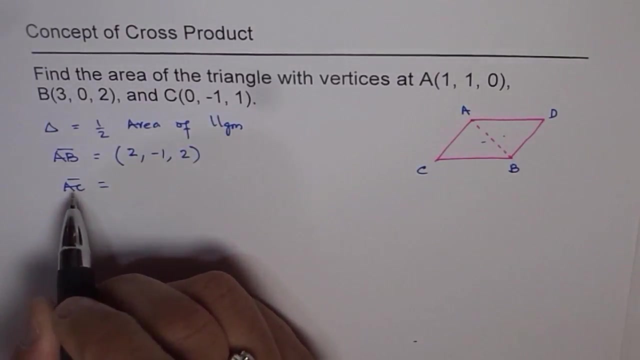 magnitude will give us the area correct. Now what is AB? A to B will be 3 minus 1,, which is 2.. 0 minus 1,, which is minus 1, and 2 minus 0 is 2.. A to C will be 0 minus 1,, which is minus 1, minus. 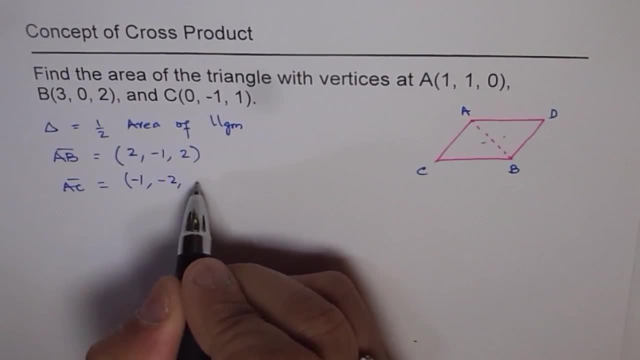 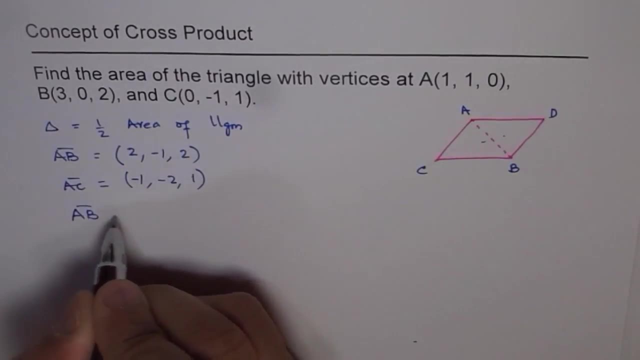 1 minus 1 gives me minus 2, and 1 minus 0 will be 1,. right, So we get AB and AC. Now what is cross product of AB and AC? Cross product of this is 2 minus 1, which is 2 minus 1, and 2 minus 0 is 2.. 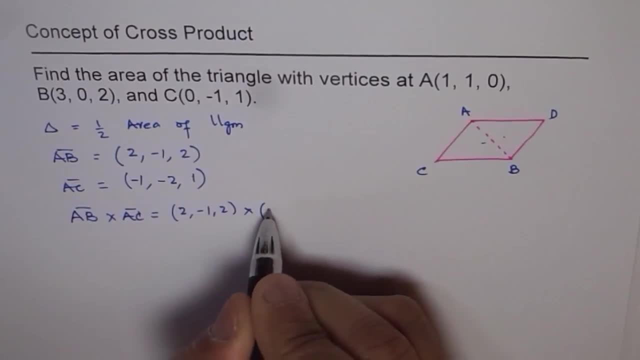 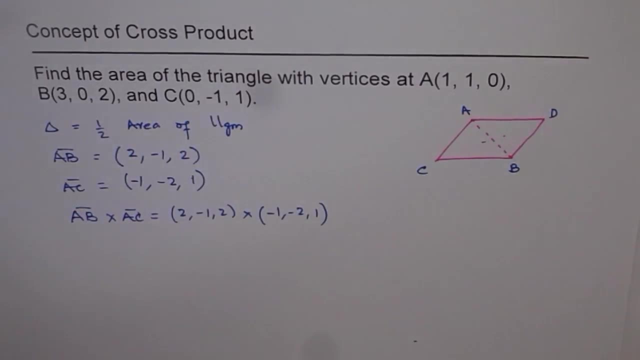 2 minus 1,, 2 cross minus 1, minus 2, 1,. right Now to find cross product. we can write these numbers in row, starting with the middle number right. So the middle number here is minus 1,. 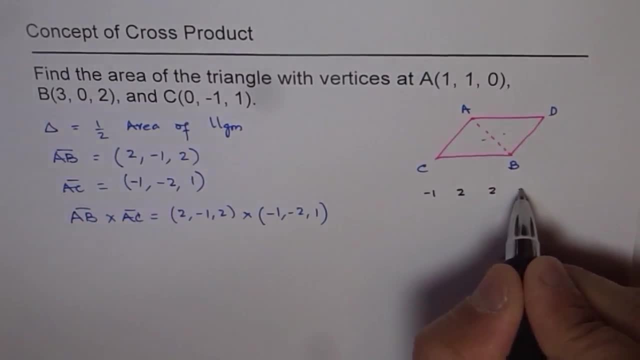 minus 1,, 2, 2, and end with the middle number. And now, here again is minus 2, 1, minus 1, and end with minus 2.. Now when we multiply, we have to add these right, We have to multiply these, and the components taken away are these: 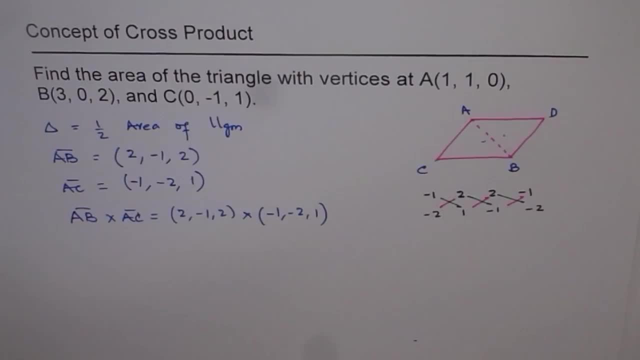 correct. So we can write down our cross product here as the I component here is minus 1, minus of 4, which is plus because minus right Plus j times. these are unit vectors: minus 2, minus 2.. 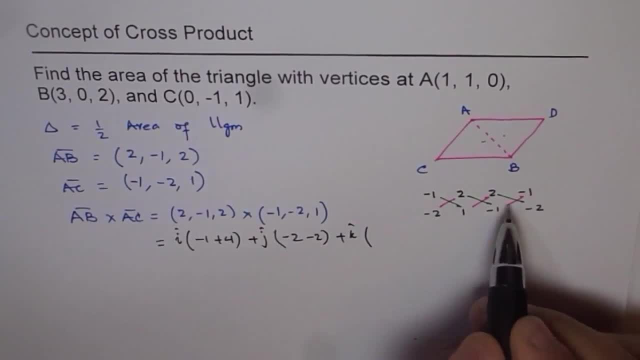 Plus k times 2 times 2 is 4, with minus sign and minus of 1.. So that becomes the component. It's a good practice to always check it right. So when you do this minus 1, and take away, 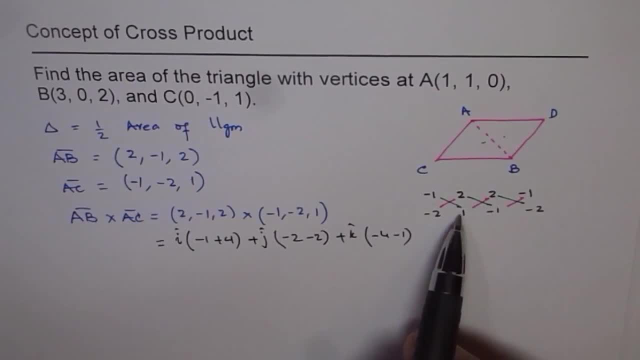 it becomes plus Minus sign first, and then minus of 2,, that's correct, Minus 4, and then this is plus minus 1,, that's correct. So we get this as equal to: i is 3, it's limited to 3i, and j component is minus 4, minus 4j and k component is minus 5,. 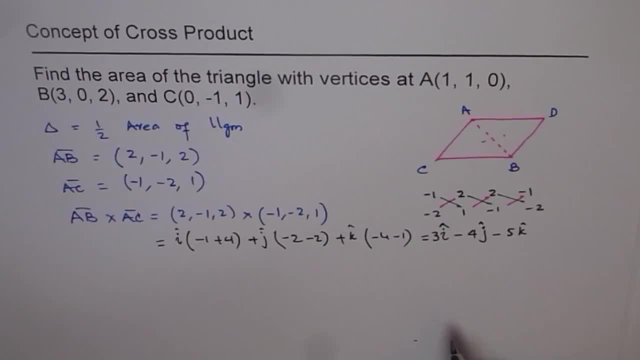 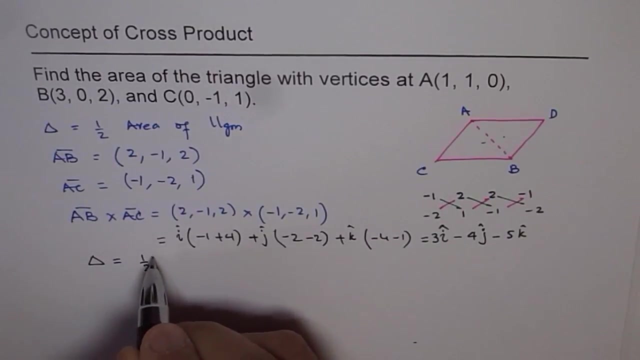 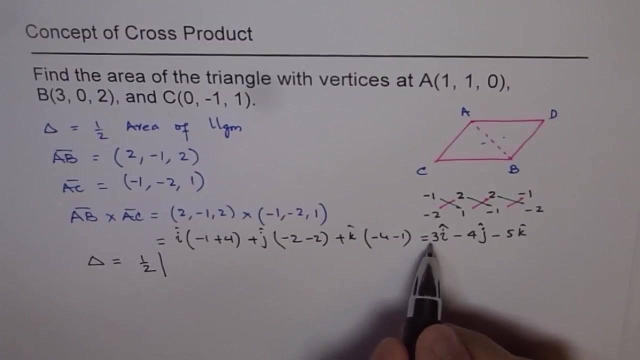 so minus 5k, right? So these are our components right Now. what is the magnitude of AB? So actually the area of triangle will be. area of triangle is half of product. of these two Scale up, I mean the magnitude of the cross product. so which is magnitude of this right? 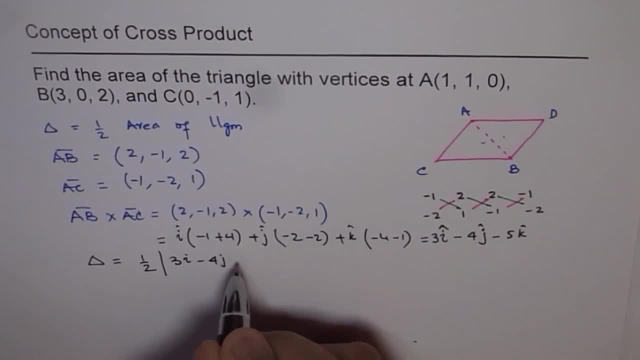 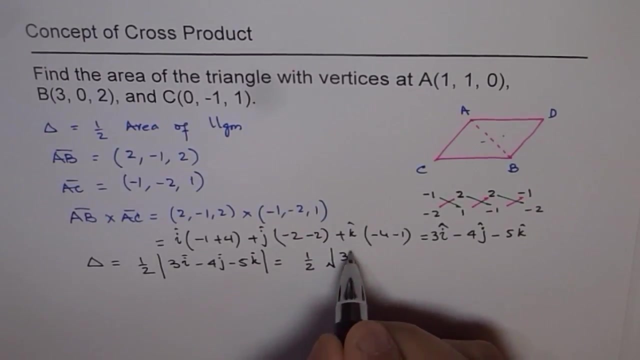 So magnitude of 3i minus 4j minus 5k, So that is your area. So this is equal to half times. so the magnitude is square root of 3 square, remember 3 square plus 4 square plus 5 square right. 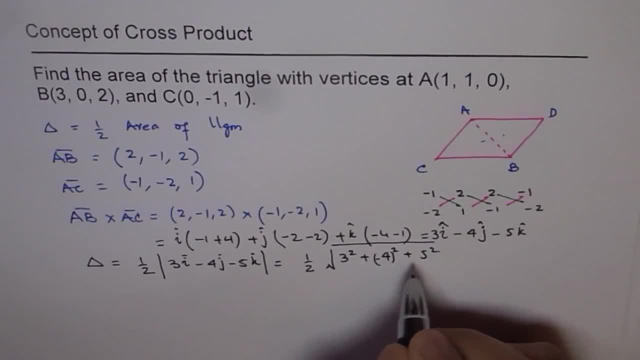 Strictly speaking, I should write minus within brackets. I know it becomes positive, but still that's the way it is right. Which is equal to half of square root of 9 plus 16 plus 25.. So that is the area, and so it is half of. we can add 9 plus 16, 25, 25 is 50.. 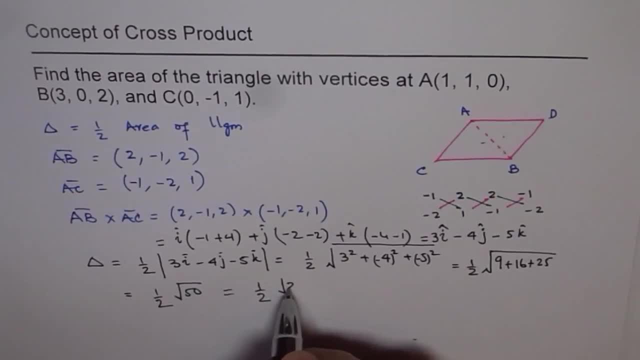 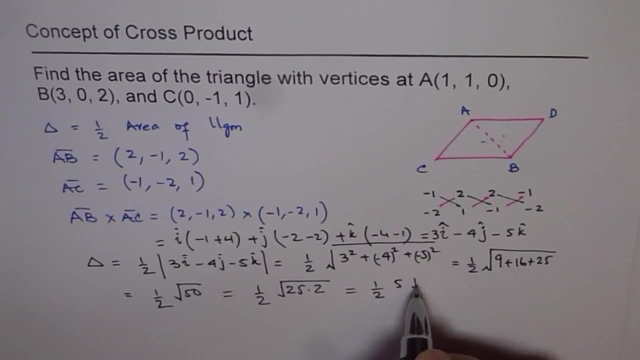 Which could be written as half of 50 can be written as 75 times 2,, so that is half of 5 times square root 2, correct. So you could write 5 over 2 square root 2, as the area in square units. 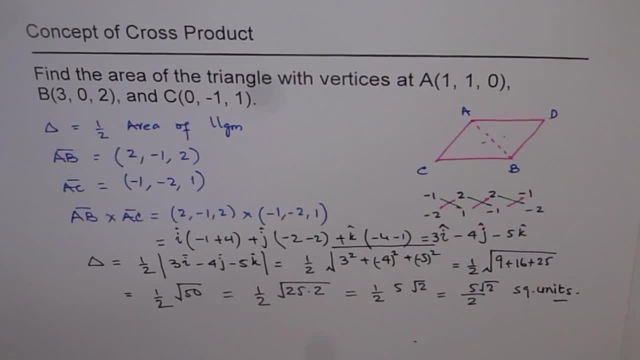 So that becomes the answer for this particular question. So I hope you understand the method. The method is: area of triangle is half the area of parallelogram and area of parallelogram and that is magnitude of cross product of the two sides of parallelogram. 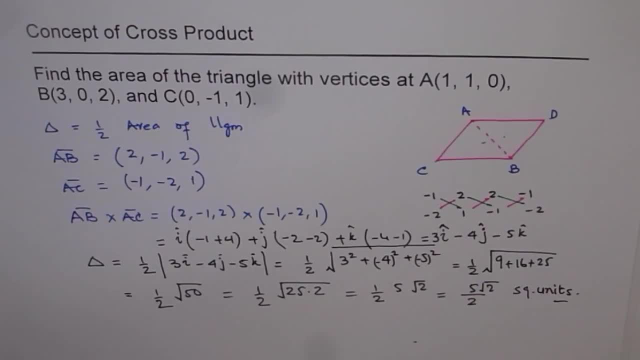 So that is, in short, the way to do it. Thank you.